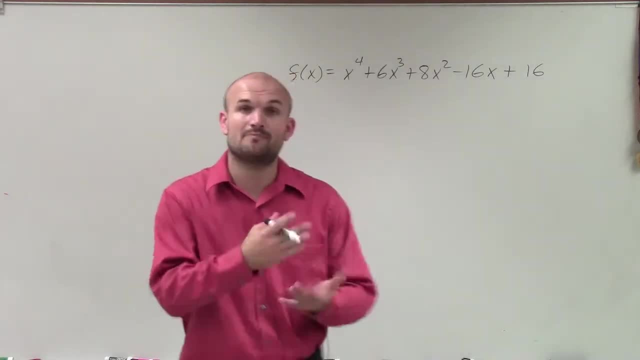 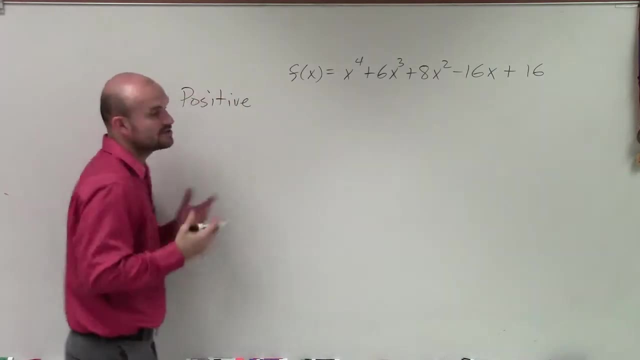 Descartes' rule of sines to determine the possible number of positive and negative real zeros. So the first thing I think is always easiest, is to take a look at the possible positive. So in doing that, what we're going to do is we're just going to take a look at the sine of our coefficients of. 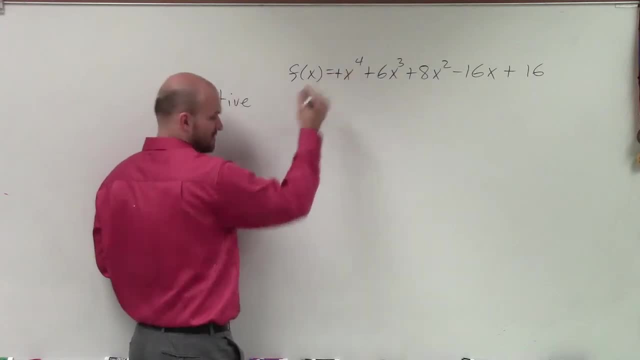 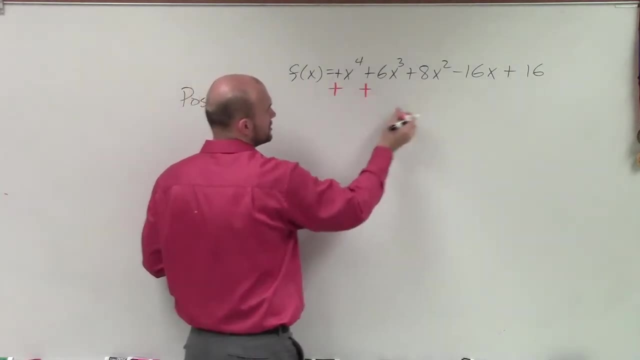 each one of our monomials. Since this is just x to the fourth, we know that's going to be a positive. Now what I like to do is I like to bring down the signs so I can see how they alternate a little bit more clearly. So I just take the sine of these coefficients out there And what you can. 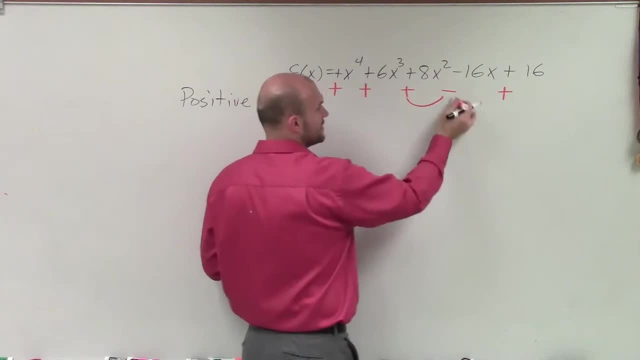 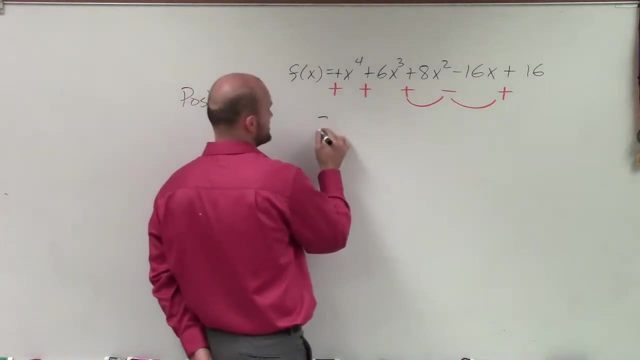 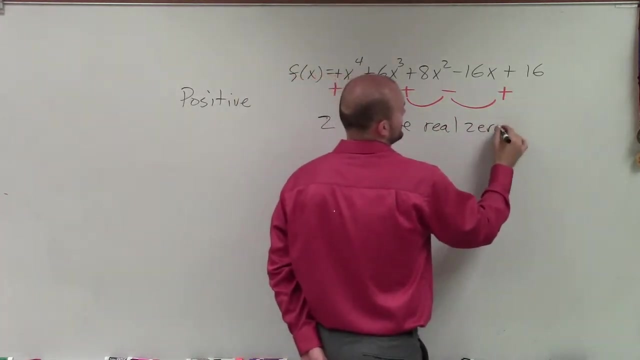 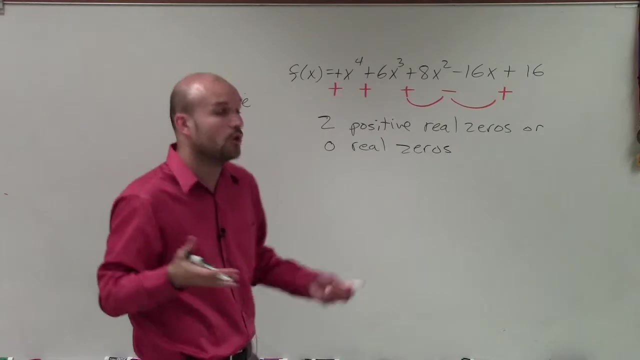 see again is there's an alternation between a positive, negative and then negative to positive. So therefore we change signs twice. So for the number of positive real zeros we have a possibility of two positive Real zeros or zero real zeros. And again, the reason why we go from two or zero is because we 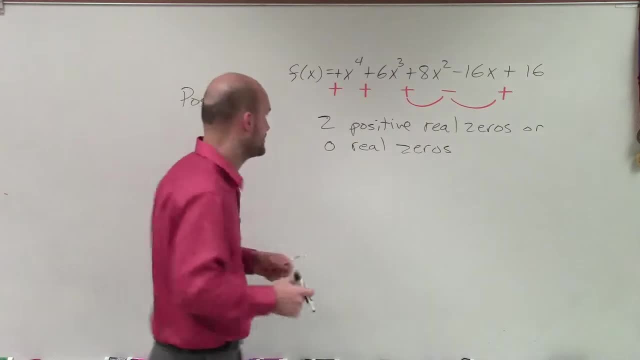 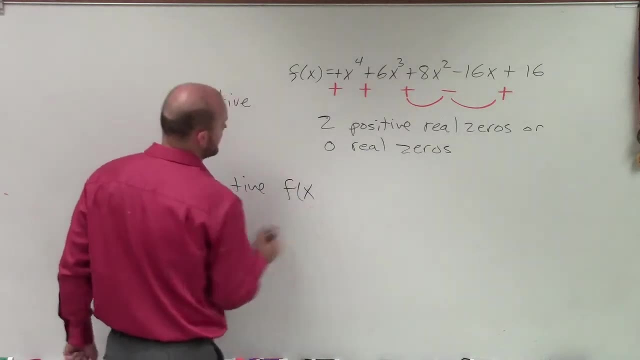 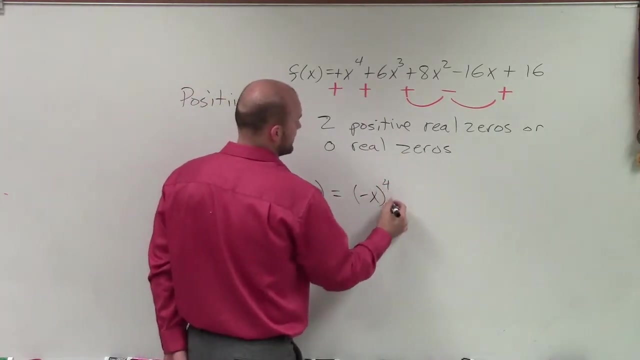 always take the number of possible real zeros and then subtract an even number Now to determine the negative. what we're going to do is now, rather than applying f of x, we're now going to evaluate for f of negative x. So we apply, so we plug in a negative x into our function. 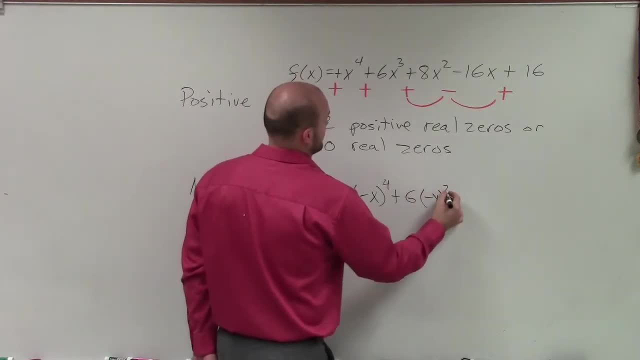 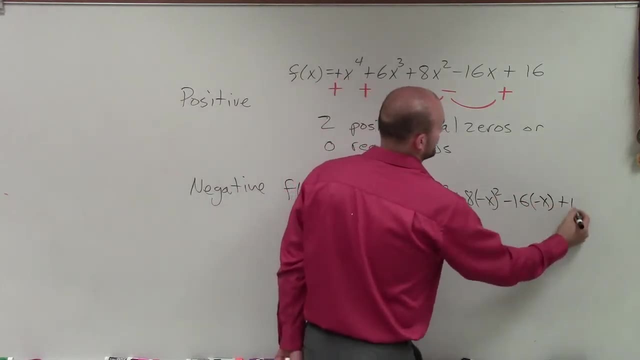 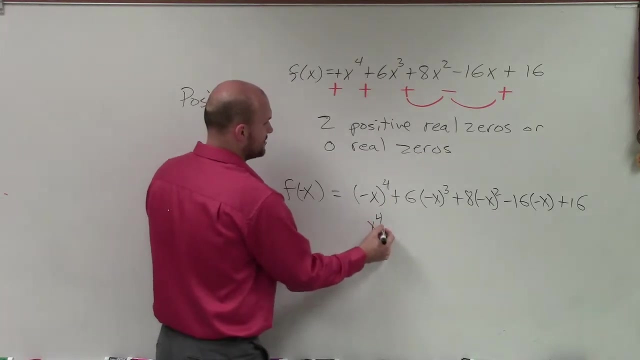 of f, of x. There's a lot of x's here. So now what we do is we just evaluate. So when we take a negative number, raise it to an even power, that's still going to be a positive x. to the fourth Negative x, cubed. 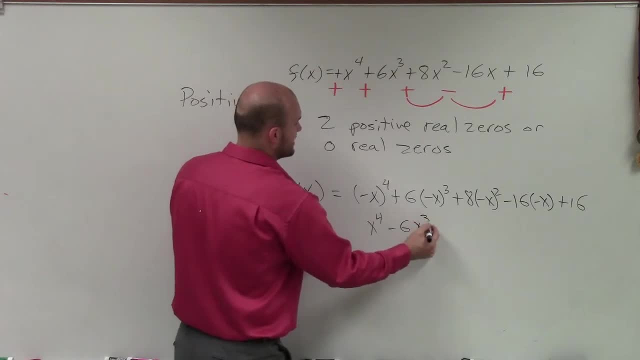 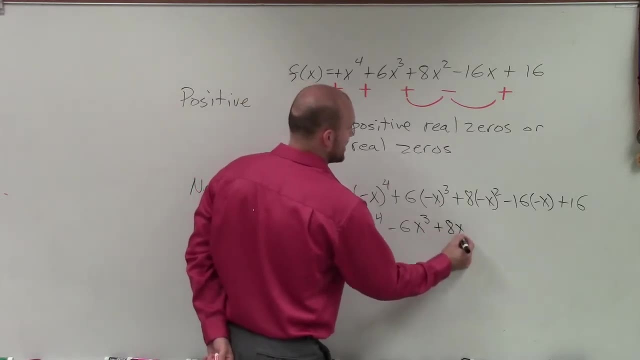 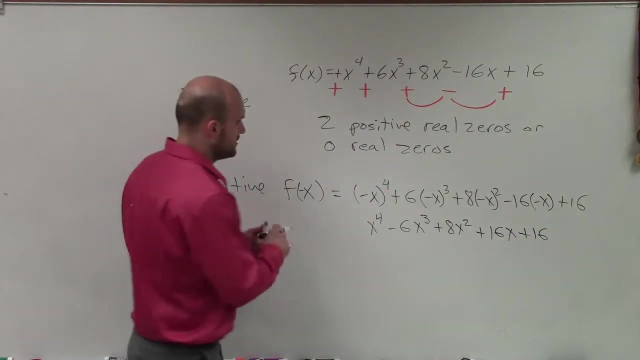 become negative. Negative times six would become a negative. six x cubed. Negative. x squared is positive. Eight times x positive. eight squared is positive. eight x squared. So we're going to. This becomes a positive: 16 x plus 16.. So now you can see again. we will bring down the signs. 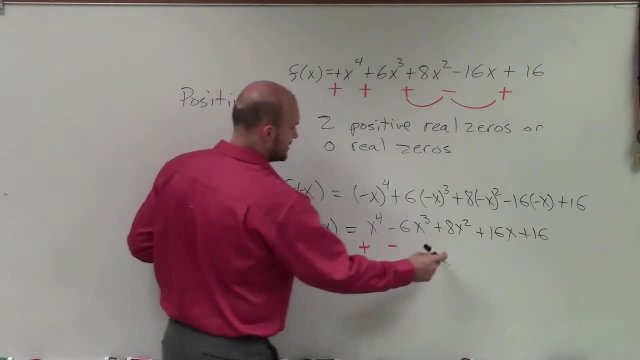 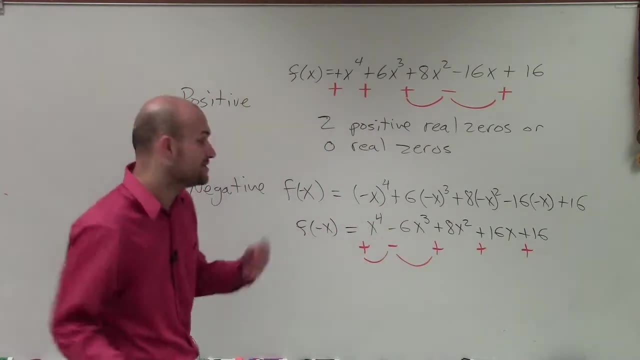 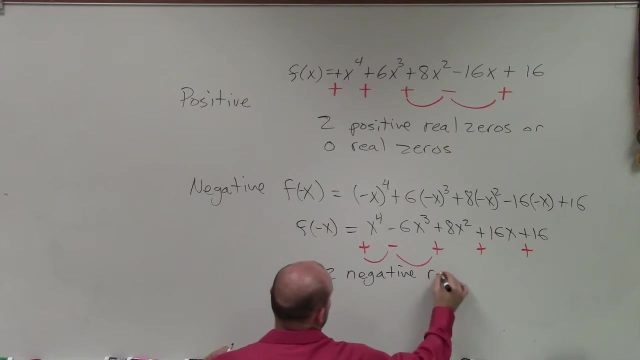 So by bringing down the signs, I know this is positive to negative, to positive, to positive to positive. So then again there's two alternating signs again. So the number now of negative real zeros is going to be two negative real zeros real zeros or zero negative real zeros.